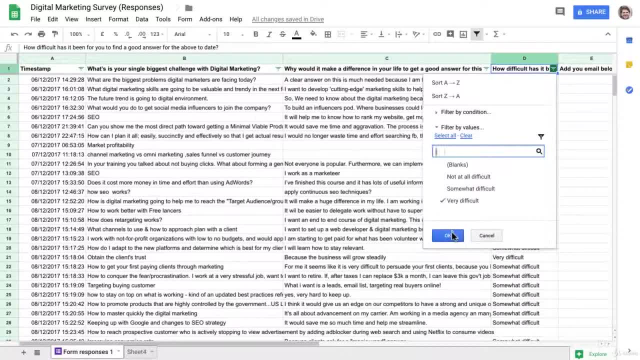 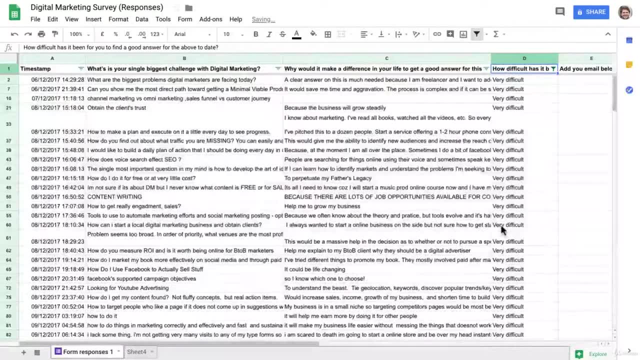 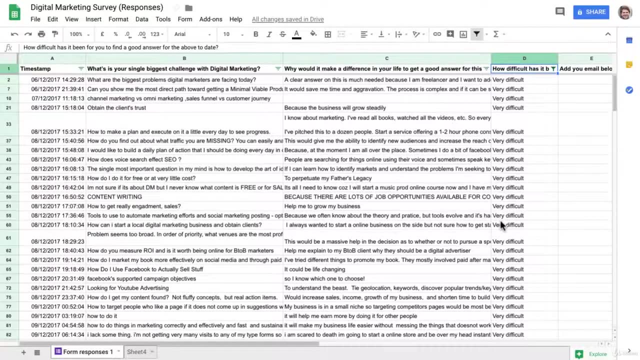 and really just look at the responses that say people have a problem that they found very difficult to resolve. Now, why are we doing that? Well, remember, if we want to create a successful product or service, or even a piece of content like a blog post or a video, we need to be solving. 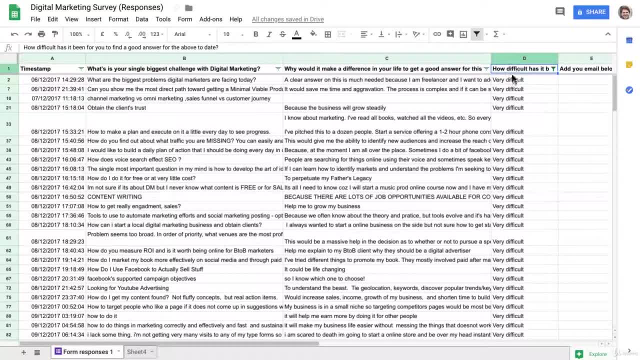 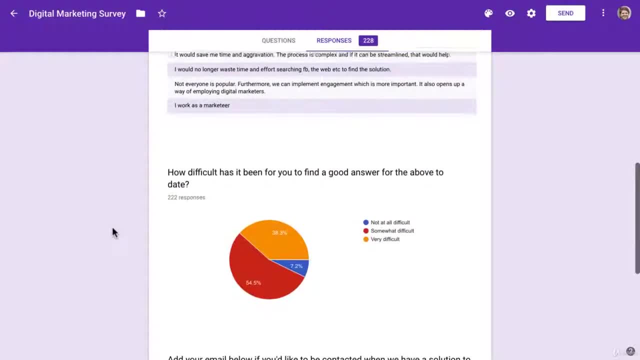 problems that are not well solved in the marketplace And that's why we really want to focus on this. And you can see, if we scroll down here just to the third response to give you a visual, we can see that around 38-40 percent of the answers. 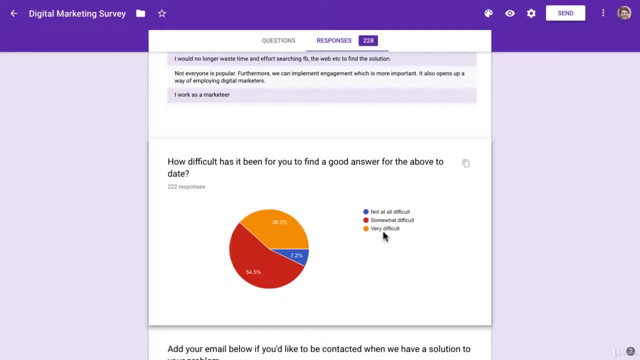 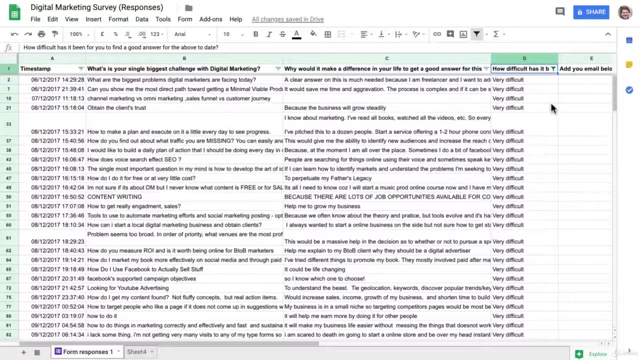 people said it's a very difficult problem for them to solve. So by just filtering that there, we have removed 60 percent of the problems that people don't think are that important or not that hard to solve, And we're just focusing on 40 percent, which for this survey is about 80 responses as opposed. 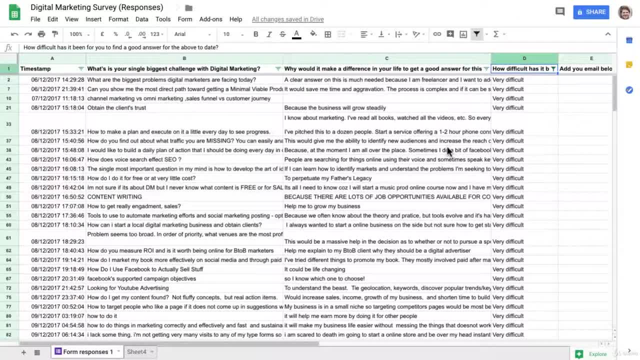 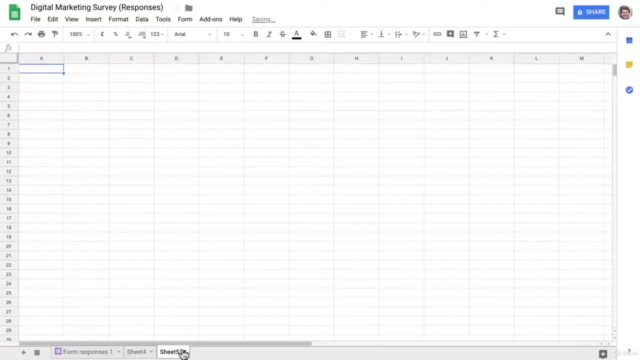 to over 200. So it just makes it easier to analyze it as well. Now the next thing you want to do is go ahead and open up a different tab here. You can just add that like that, What we're going to do in this tab is just write down problem. 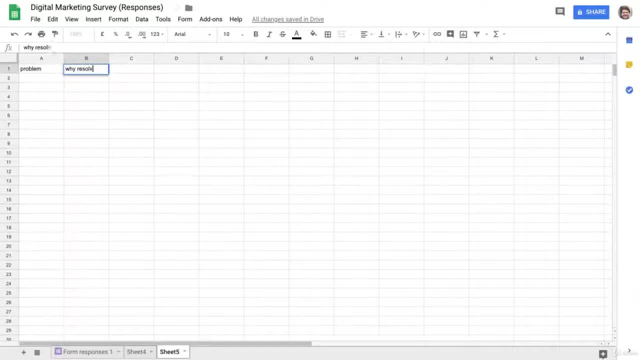 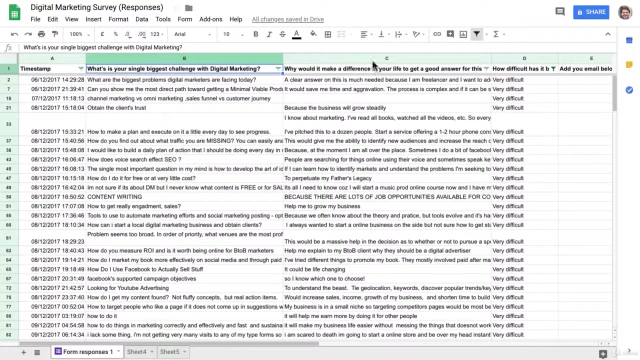 and why resolve it. So these are the two important things that we want to get out of this survey. when we look at it, We want to know what the problem actually is and why it's going to be important for them to resolve it. So that will really come from these two columns. 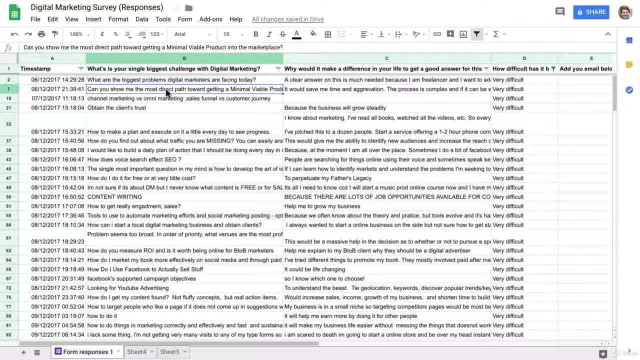 So let's just go and have a look at it here. So, OK, Not every response is going to be perfect, so you're going to just have to go through one by one, down through them and pick them out. So let's see the problem here. What's your biggest challenge? Can you show me the most? 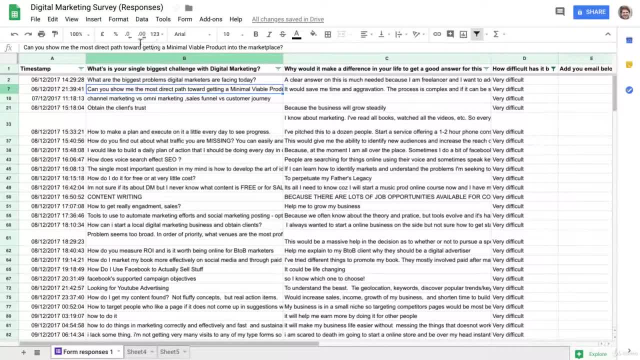 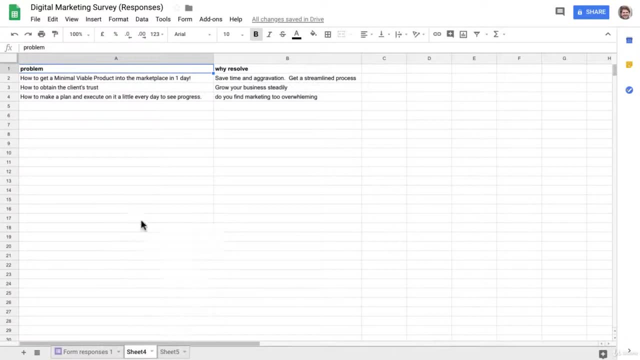 direct path towards getting a minimal, viable product in the marketplace. OK, So that's a great problem to solve. So what we can do is: I always like to frame the problems as like a how to. I'm going to delete this one I did earlier so we can start fresh. 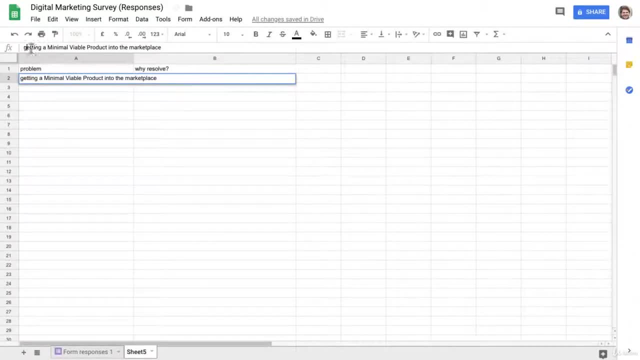 And what we can do is just pop this in. And what I like to think about is, if I was writing this as a course or a piece of content, like a blog post or a YouTube video, what would the title be? It's always just easiest to start with how to, So how to get a minimal. 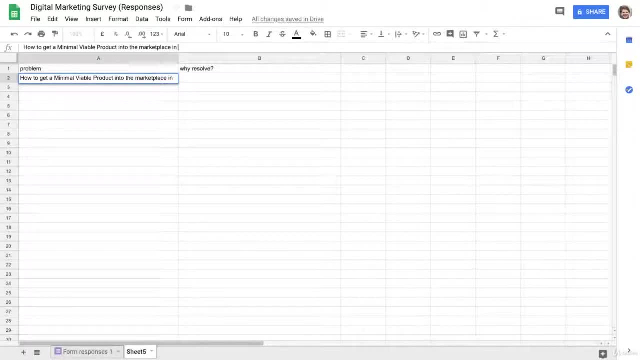 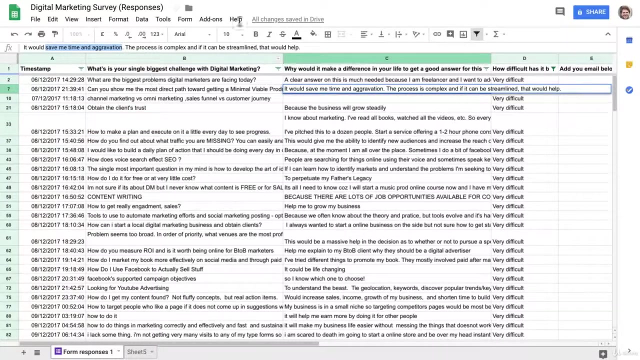 viable product into the marketplace, Let's say in one day, because they're looking for speed. That's what they said in their response here. Let me go back to this tab. OK, It would save me, save time and aggravation. So that's a. 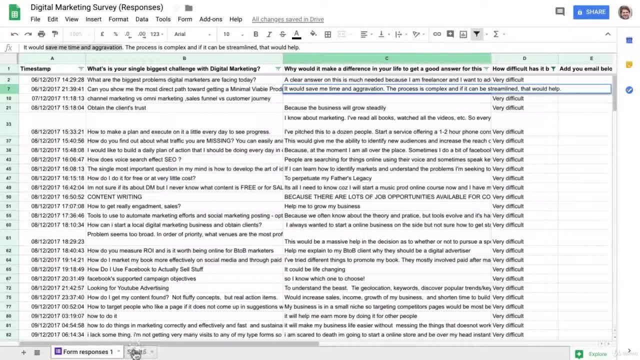 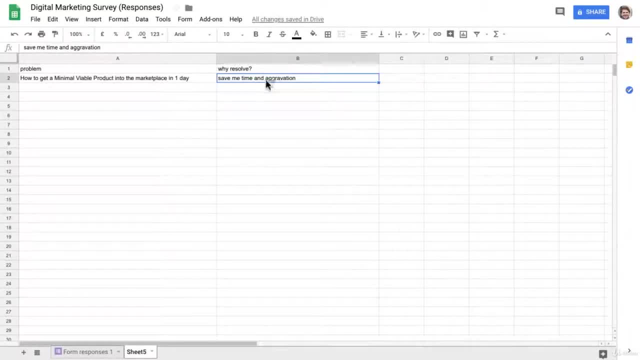 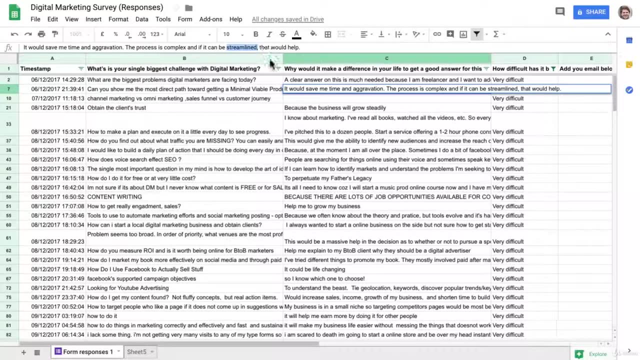 benefit. I'm going to close this down, actually, because I keep clicking back to it, So you know why would they, why do they want to resolve this, Why would they buy our product or read our blog post? to save time and aggravation, And they're really looking for a streamlined 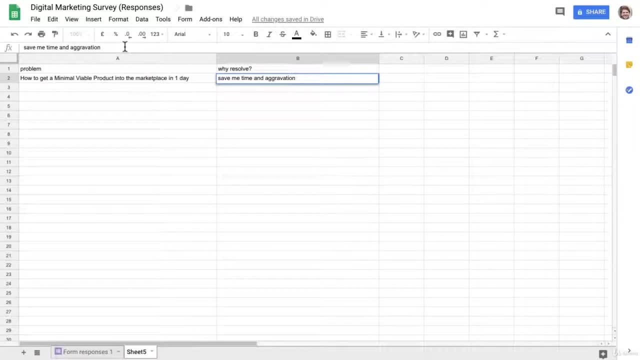 process. So that's another benefit of them maybe buying our product or service or reading our blog post. So get a streamlined process. So you can see already here, just reading one response, What I've got for me is a potential course that I could make, or even a potential section or lecture within a course. a potential 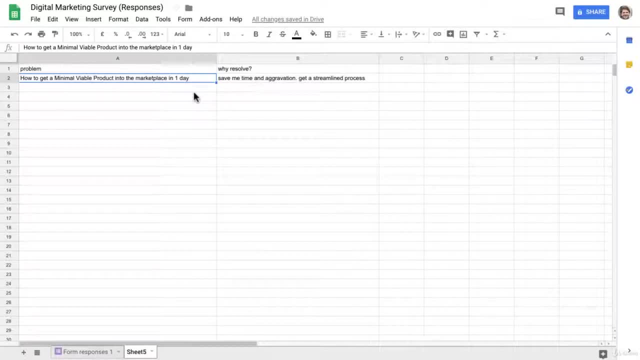 blog post a potential YouTube video that is tailored to my audience And that would really resolve a problem that they have. What are some of the benefits that I could mention? at the start of that video, or course, or put on the sales page or in a Facebook ad: Look, this is going to save you time and 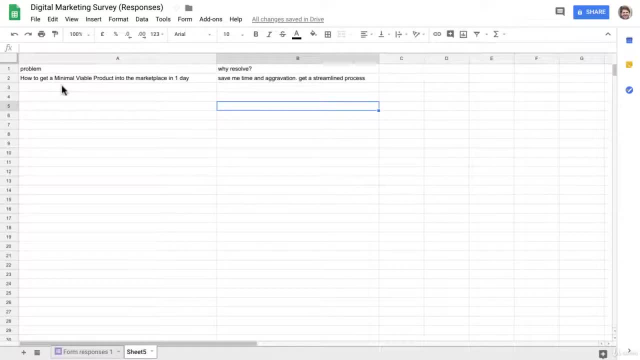 time and aggravation, you're going to get a streamlined process to get a minimal, viable product into the marketplace in one day. that's a very good pitch and offer and it resolves a pain point that people have. so that's only one answer. now let's go down and have a look, okay. 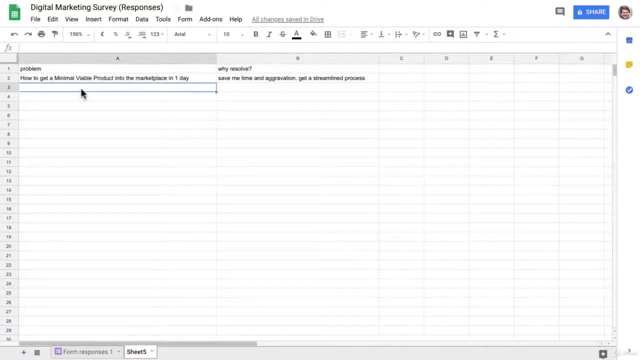 what we can do. again same process. i'm just going to do three of these to give you examples of what you should be looking out for, and then, obviously, your responses are going to be different. so how to obtain a client's trust, i guess, as a digital marketer, is really what they're asking. 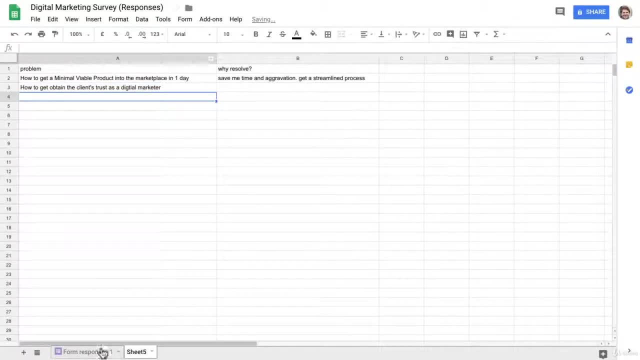 here, and why would they want to do? to do this, you know, grow your business steadily. that's what. that's why they want to resolve this: because they think trust is a big barrier to signing clients. and that's true. how can you get them to trust you? they're going to hand over money and access to you know their 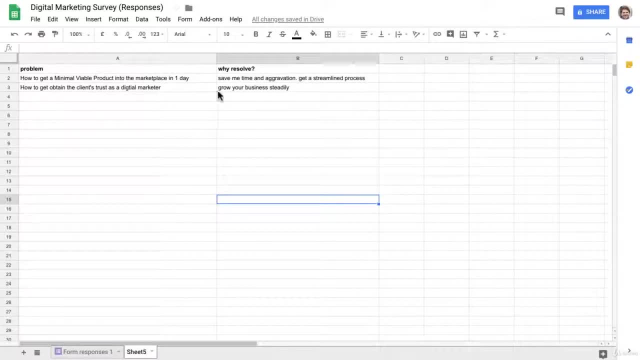 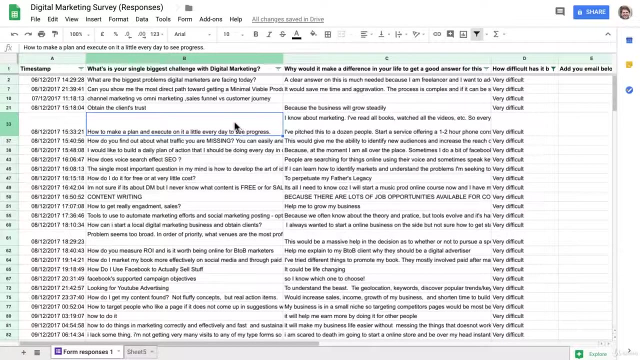 analytics or whatever. so this is a big barrier for a lot of people. how do you overcome that? that could be a great lecture or a course or a blog post or whatever could be a great something piece of sales copy on a course or facebook ads. so, again, you just just copy and paste. this is 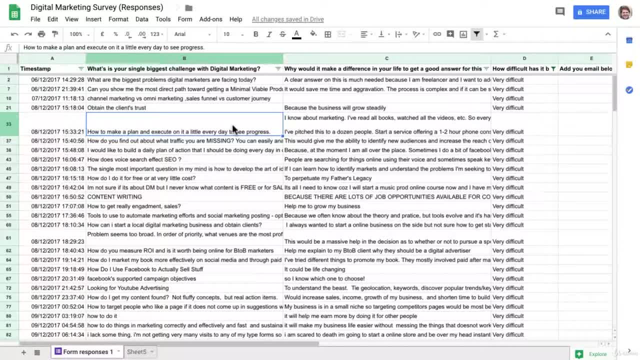 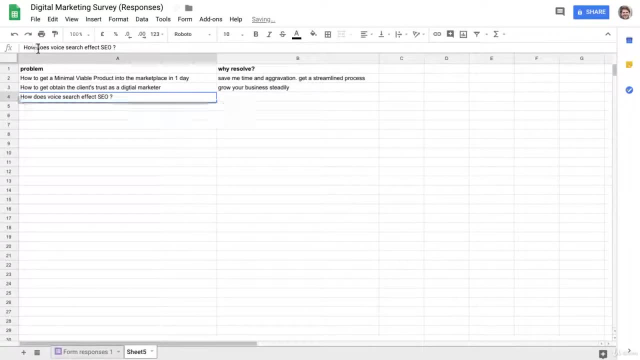 why this process is so beautiful and powerful, because there's very little work for you to do once you start to analyze it. so let's have a look here. this looks interesting. um, how does voice search affect x seo? this could be something interesting. you know how to. 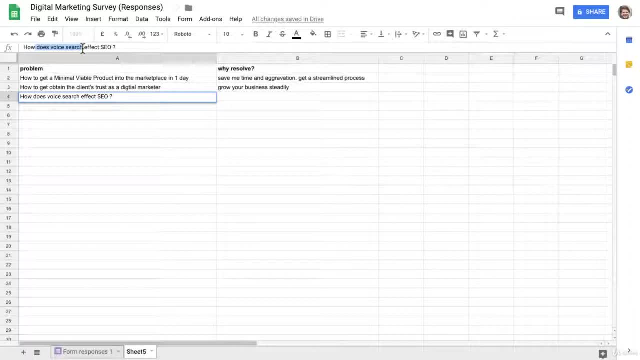 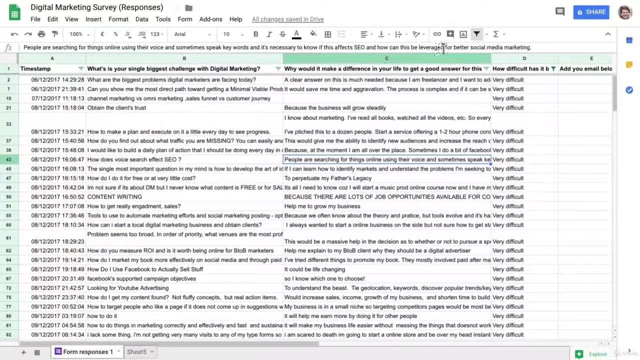 how to benefit from voice seo, maybe, or how to rank number one from voice seo on mobile, let's say, for example. so i'm just thinking about you know what does the how to look like to resolve that problem and why would they want to do this? you know, leverage voice. 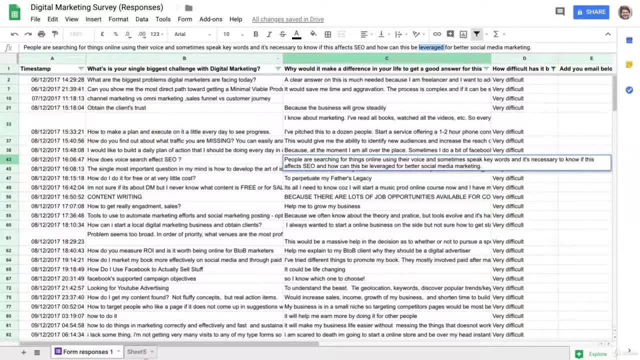 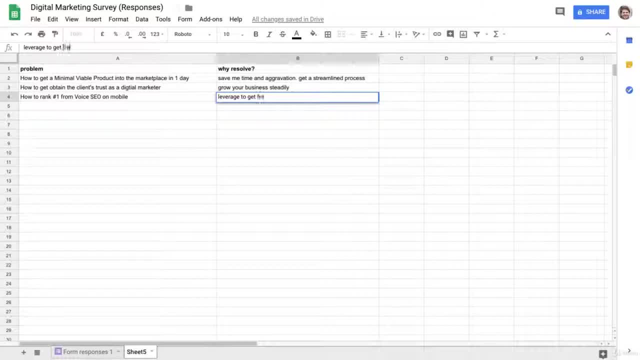 leverage voice, voice seo. to get to the leverage voice seo, i know why: to get free traffic to your site. so you can see i'm i'm using what i'm hearing from the customer here and adding, how you know, putting my spin on why they would want to do that. and this allows me just looking at.